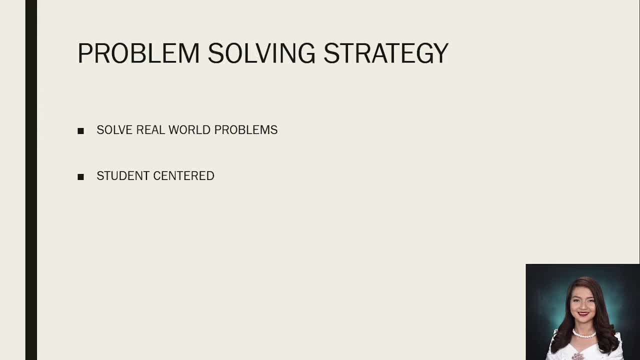 or the problem solving strategy, is the time given to the students to struggle with the problem, and its beauty is in the varied solution that the students would produce. Problem solving skills help you determine the source of a problem and find an effective solution. Although problem solving is often identified as its own separate skills, So there are other related. 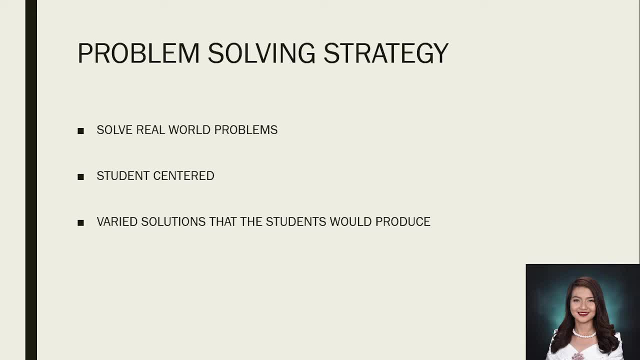 skills that contribute to this ability. So some key problem solving skills are active listening, analysis, research, creativity, communication, dependability, decision making and team building. So problem solving skills are important in every career, at every level and also, if you're. 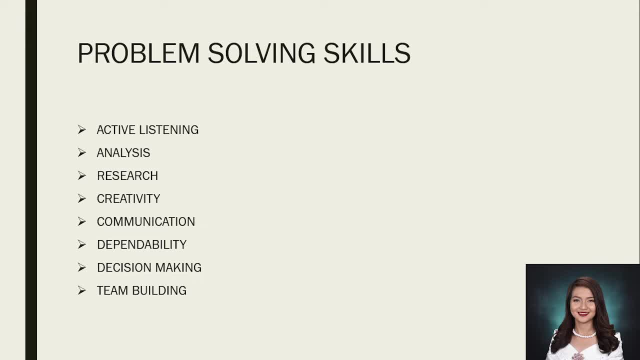 teaching, especially when you're teaching those primary grades. So, as a result, effective problem solving may also require a good in this industry or job, specific technical skills, for example. so to solve a problem effectively, you will likely use a few different skills. so here are a. 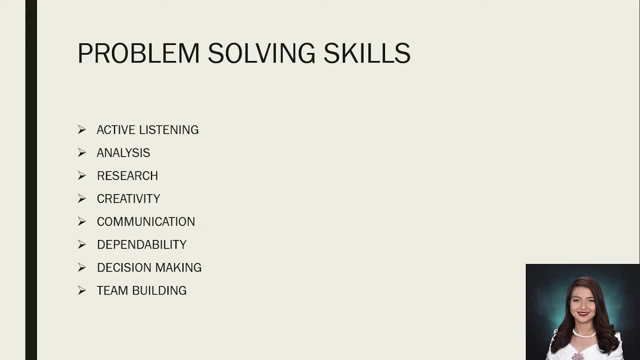 few samples of skills you may use when solving a problem, for example in research. so researching is an essential skill related to problem-solving. so as a problem solver, you need to be able to identify the cause of the issue and understand it fully. next is, for example, we have here the decision-making. so 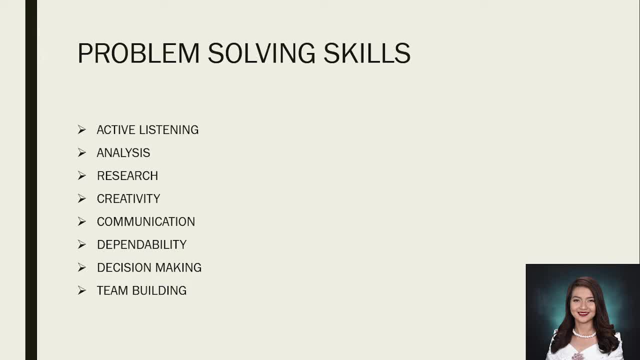 ultimately, you will need to make a decision about how to solve problems that arise. next is the communication. so when identifying possible solutions, you will need to know how to communicate the problems to others. so, in improving your problem-solving skills, there are several methods you can use to. 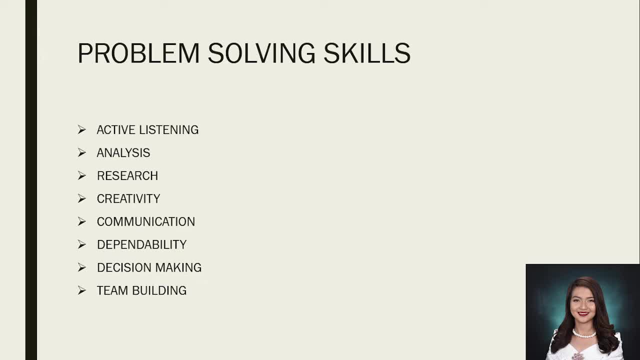 improve your problem-solving skills. so, whether you are searching for a job or currently working, improving your problem solving- and also in improving the problem-solving skills, especially when you teach, you can practice them and also you can have the role play, so it can be useful tools when learning to develop. 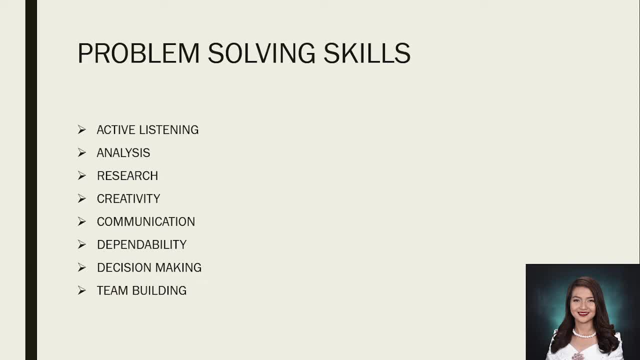 their problem-solving skills. so you can find also professional practice books and problem-solving scenarios, even in online. so practice how you might solve those problems and that they mean if your potential solutions are viable. so let's proceed to the three main elements of problem solving. so let's proceed to the 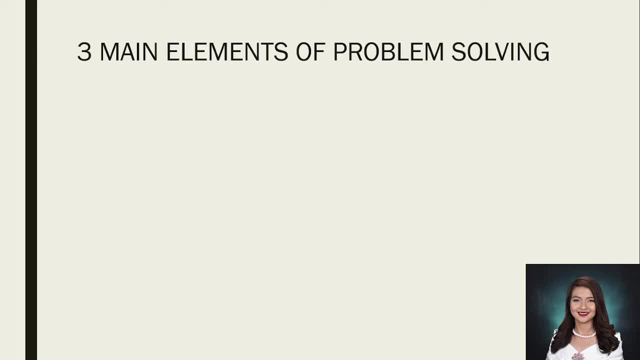 main 3 main elements of problem solving. so first we had the word problem, next is given for the students to struggle with the problem and lastly we have the mathematical discourse that happens during the struggle and during the processing of the student generated solution. first let's talk about the word problem. so in many filipino classroom word problems are: 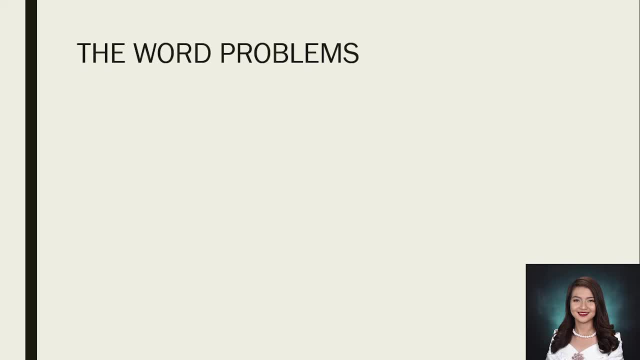 given at the end of the lesson and the students are expected to answer them by applying the concepts or skills that just had been taught to them. so in most cases, the teacher first demonstrate how to solve a problem and then the students would independently answer a similarly structured problem. so in this practice the students are not doing problem solving. they 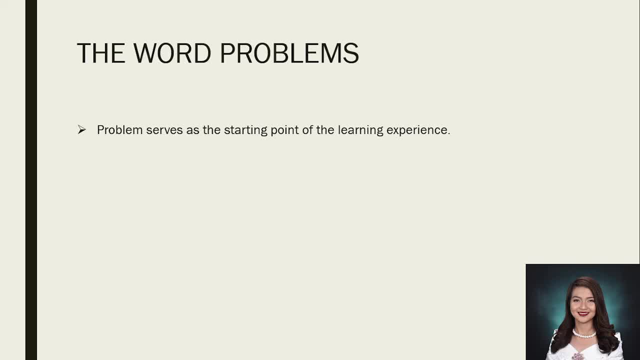 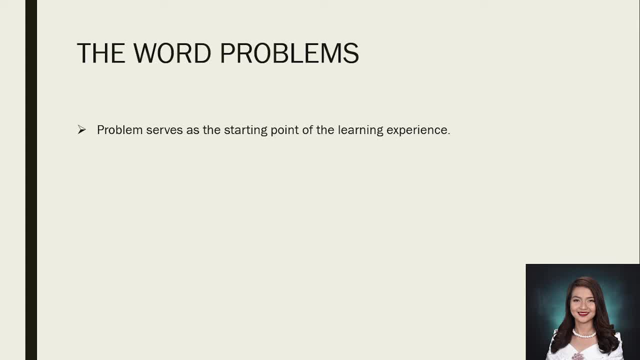 created a problem which can be originally solved and also answered using previous the crash-cami knowledge and skills. so how you present the problem also matters, personally for the primary grains. so it is not always helpful to introduce the problem by posting it on the board. you should not only post it on the board but though. 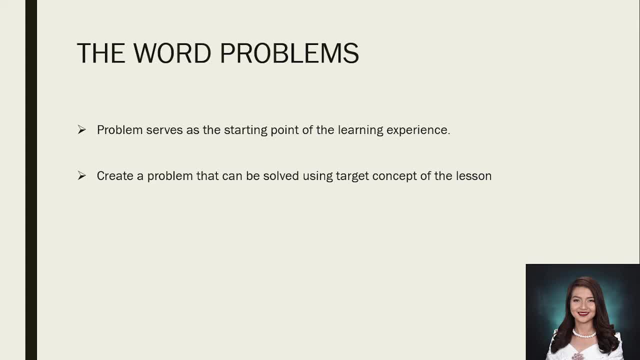 This may intimidate some students and reading and comprehension skills may intervene, because if you post it already on the board, they will feel nervous. So, instead of posting it on the board, encourage the students to imagine the scenario and allow them to clarify the information If they find some details confusing. showing drawings or real objects might help. 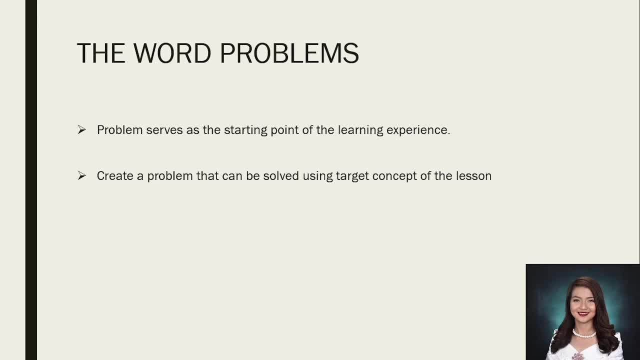 So you can use some drawings and also some illustrations. or also you can use different instructional materials before presenting it to your students So that they will feel nervous. They will not feel the nervousness and it will not intervene their reading and comprehension skills. So you can also narrate the problem in storytelling manner. 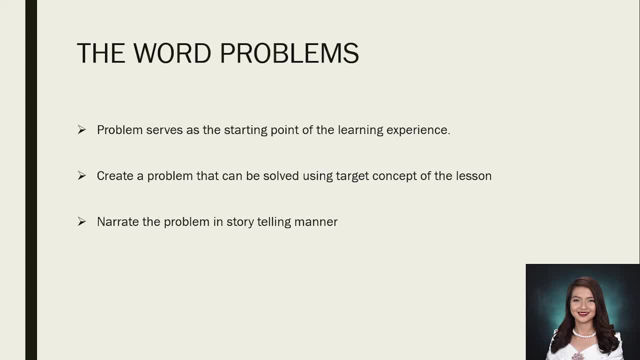 It is suggested to narrate because it can engage the learners. You can tell them a story before presenting the problem. So, for example, they love candies. You can have some examples. You sing those stories so that they will participate in your discussion. 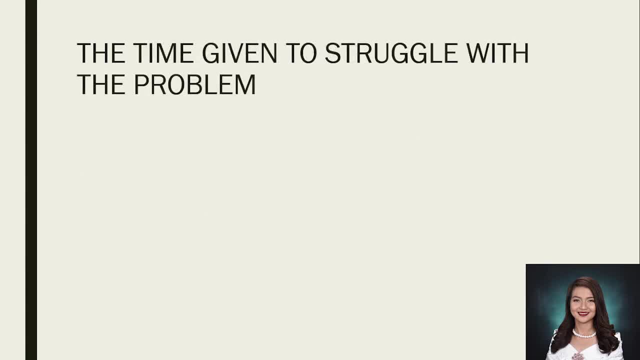 Next is the time given to struggle with the problem. So the goal is for the students to collaborate, share their ideas with each other to come up with a solution. So you must encourage the students to use their previously learned knowledge and skills to solve the problem. 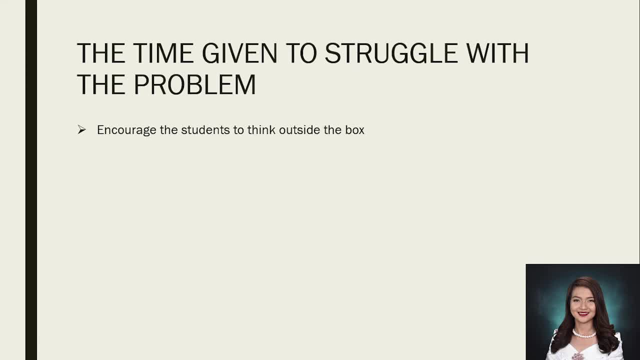 and to communicate their ideas with their classmate through words, equations or illustration. So you must encourage also your students to think outside the box. So it is natural for the students to find this phase burdensome, especially when it is the first time to engage in such an activity. Task of the. 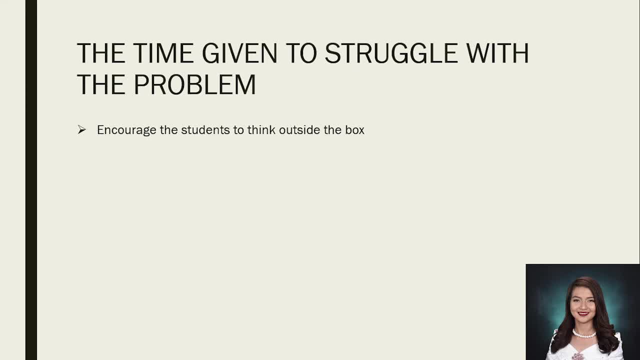 teacher to encourage the students to think out of the box. So tell the students that there is one. there is more than one way to solve problem. They do not need to worry about their solution being wrong as long as every step they did is meaningful in solving the problem. So you must. 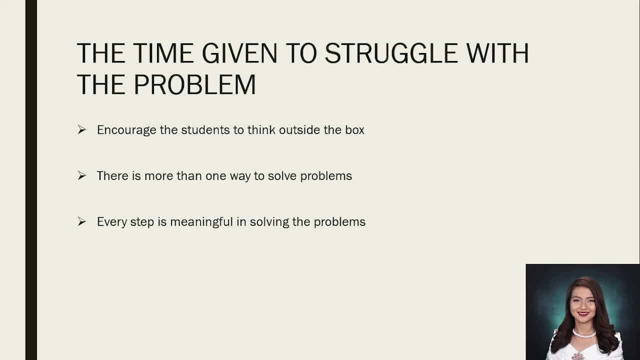 not teach them one solution only or one step in solving the problem. You must encourage them and show them the different ways on how to attack or on how to solve those problems. Next is the mathematical discourse. This is the most exciting element of the problem solving. 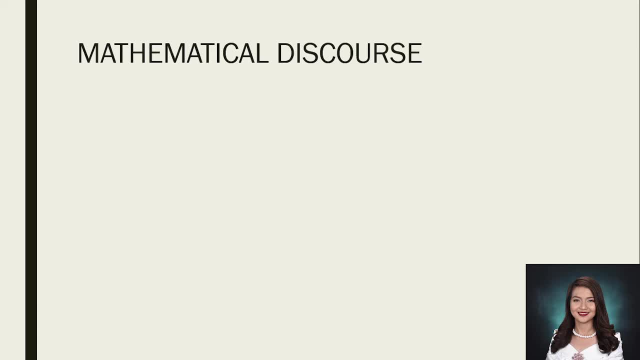 strategy. So a discourse is a spoken or written communication between people, especially serious discussion of a particular subject. The students are working in small groups to solve their problems. You get to move around and enjoy the mathematical talk. the students are engaging in discussion when correction and clarifications are needed, but be careful not to give hints. let them 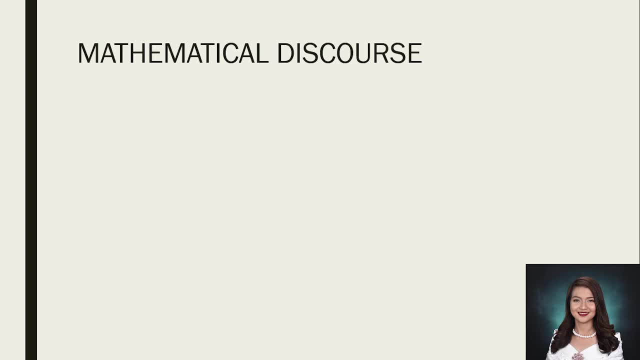 answer those activity. you just you're just going to instruct, you're just going to facilitate, you're just going to help them in arriving, in arriving. those may be tempting to do, especially when the student is struggling, but do not assume, courage your students to think, believe that they actually. 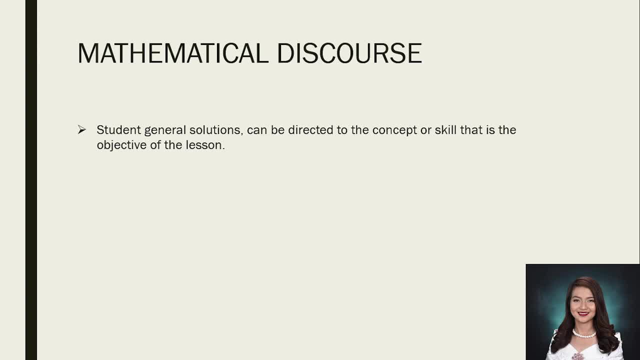 can solve, to be amazed at how the students would defend their thinking, correct each other's ideas and figure things out on their own. general solutions can be directed to the concept or skill that is the objective of the lesson. this phase camps the importance of the teacher's fluency. 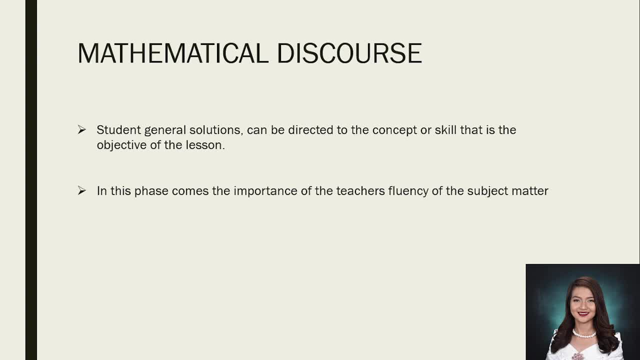 of the subject matter. so the challenge is: how would you process those by various solution, make sense of each them and use them, generalize or come up with solution that make use of the knowledge skills? that is the objective of the lesson summary. a good use of the problem solving strategy involves 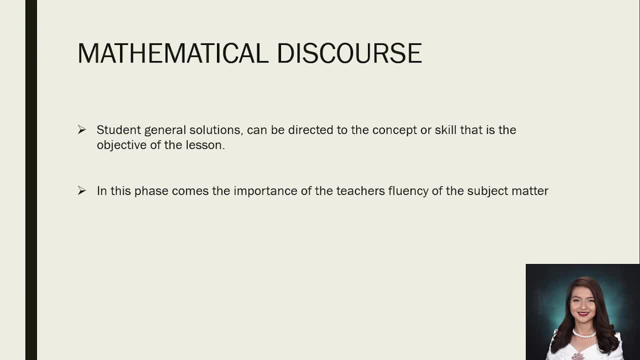 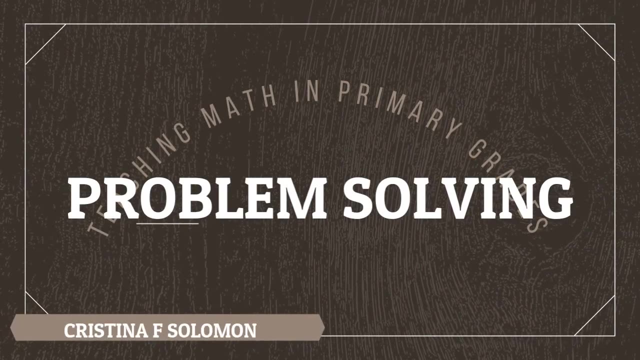 a realistic problem, ample time for students to think about the problem and a venue to engage students in mathematical discourse. so that's all, sweetie. see you in the next video. bye.